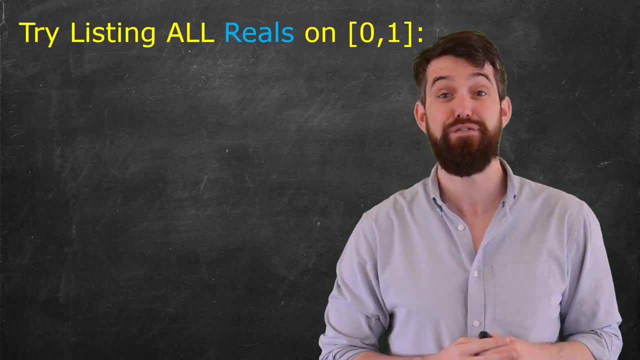 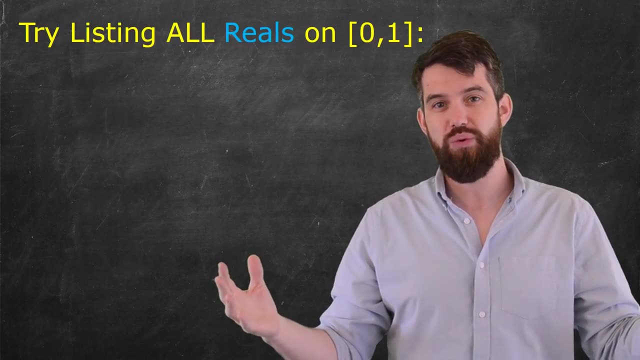 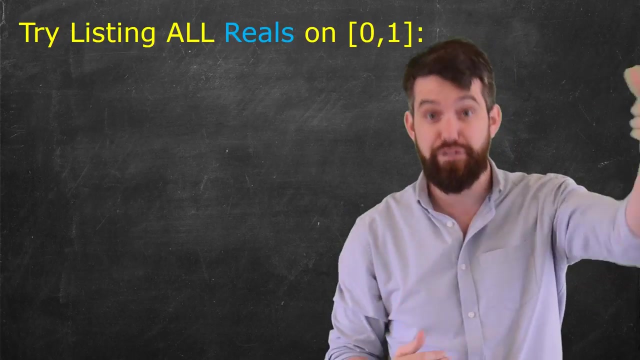 The real numbers had the same size, then we could find some function. We could line up the integers and the rationals and we could pair them in this bijective way. So what I'm going to do is I'm going to try to list all of the different real numbers. Let's just make an infinite list. It'll be a first. 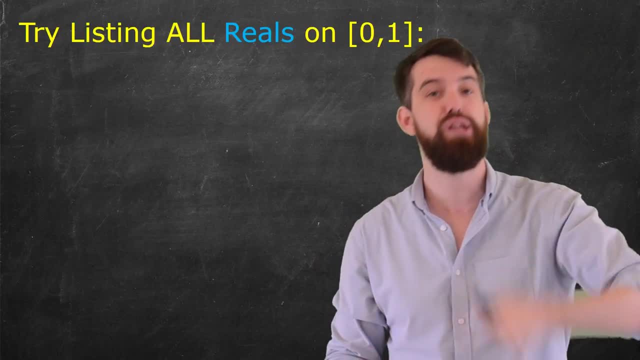 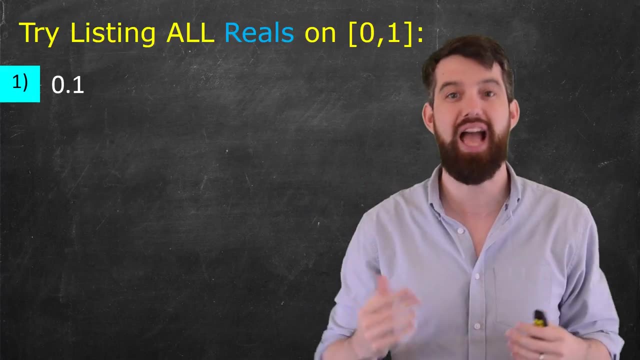 a second, a third and a fourth lined up with the first integer, the second integer, the third integer and the fourth integer. Now I'm going to sort of make up which of these real numbers I want to go. first and second. They could be anything. How about the first one could be 0.1?. 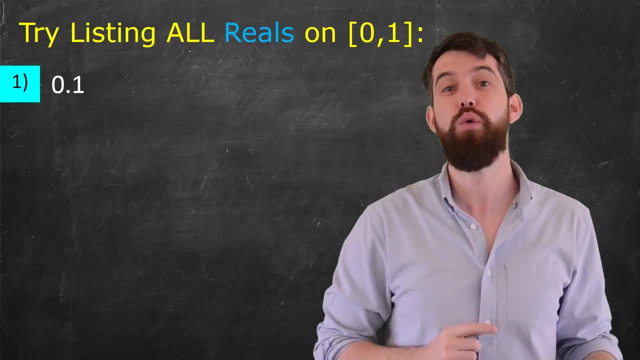 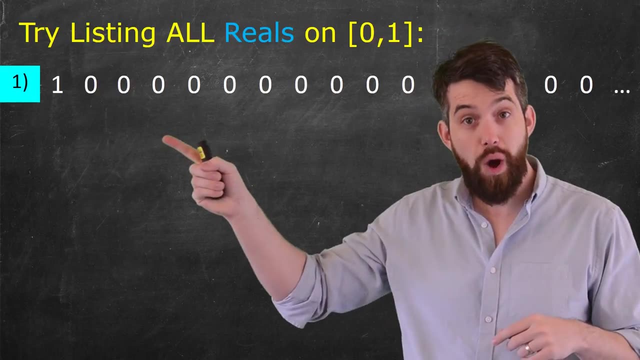 That's a real number in between 0 and 1.. I'm actually going to go and write it in terms of its decimal expansion after the 0 point, So this looks like a 1 first and then all the rest 0.. 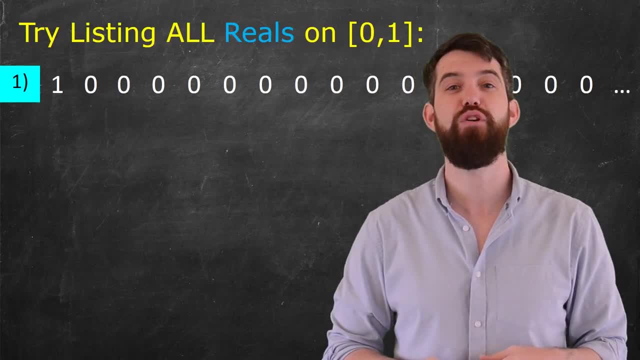 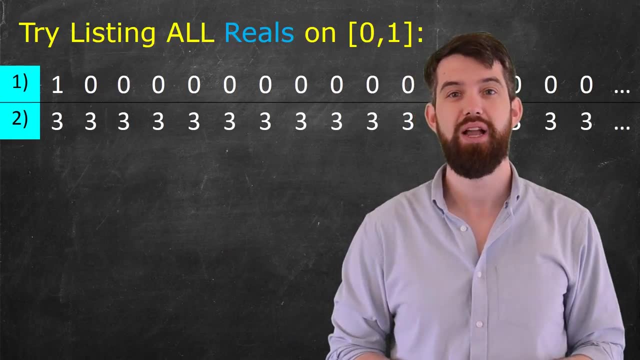 0.1000.. Okay, how about for the next one? I'll do 0.3333333, a decimal expansion for a third. It's another real number. Then I can do 0.14159265358979322,. 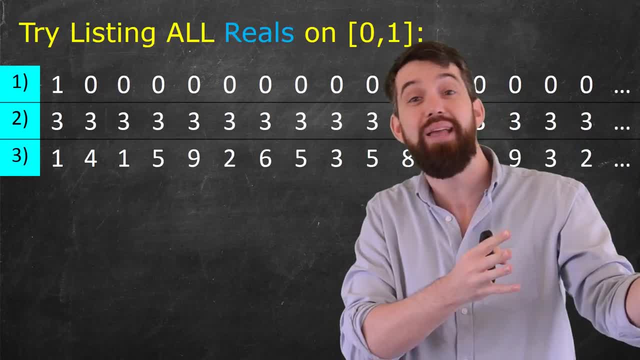 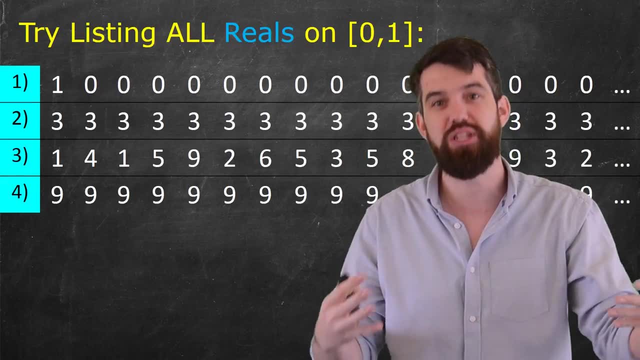 which is the first bit of the decimal expansion for pi minus 3.. It's just kind of fun, I'm just putting some random ones in there. How about 0.99999, so on? This is a decimal expansion for the number 1.. And then I'll fill up with 1- 7th, 2, 7th, 3, 7th and 4- 7th, which have some cool. 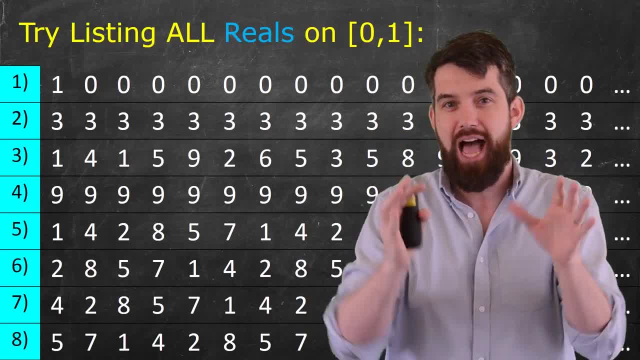 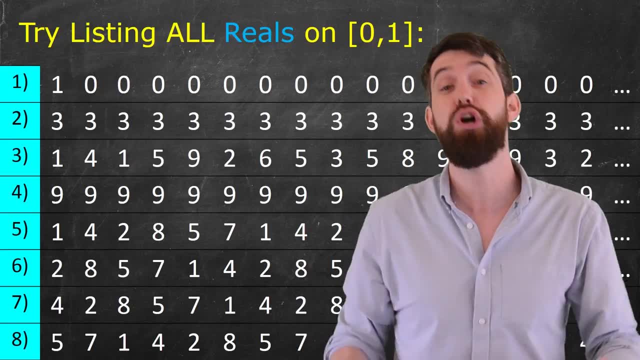 patterns, You can see how that works, But the point is this: I've just chosen these at random. You could choose whatever ones you wish, and any other real number that you might imagine we're going to suppose could occur on this list. 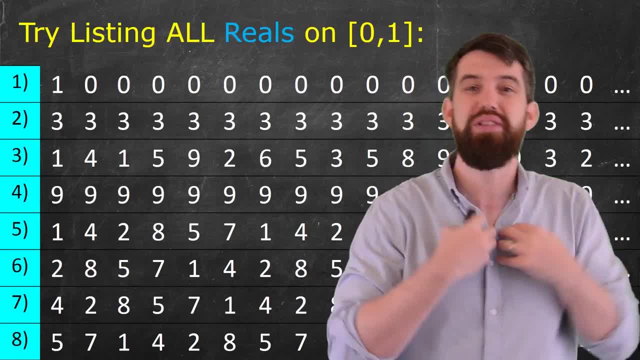 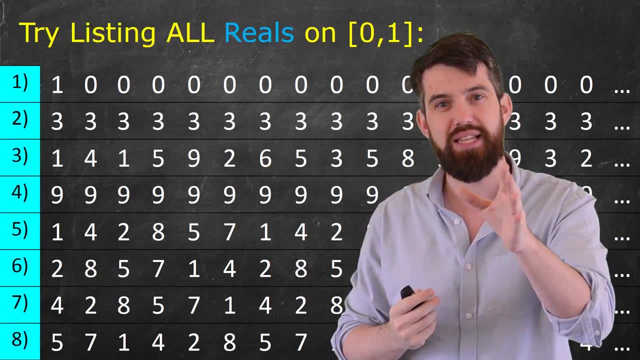 But what I want to argue is that, no matter how you did it, no matter what choices I made or what choices you made for how we tried to line up the real numbers and the integers, no matter how we did this, that we could not get all of the real numbers. So now I want to draw your attention to 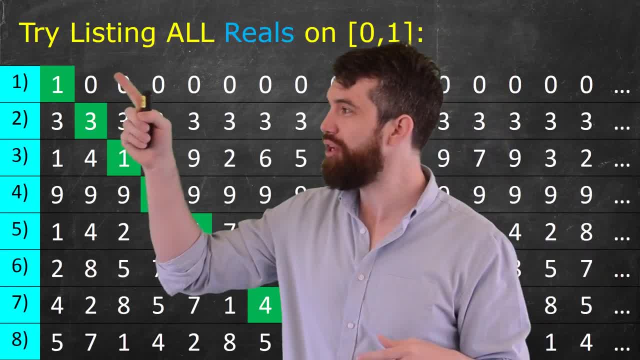 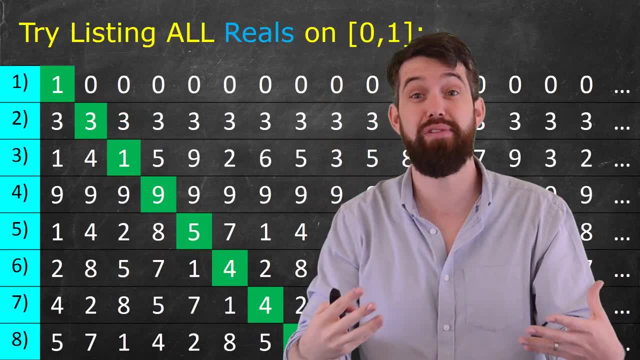 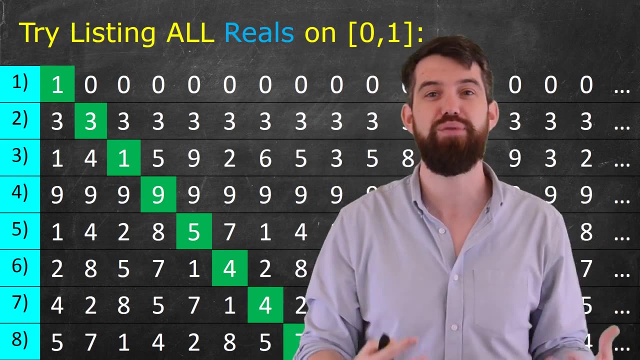 these so-called diagonal entries. It's looking here at this first digit, the 1- 10th spot, in the first particular row, the first real number we've identified, and then it's going to go down and look at the second digit in the second real number, the third digit in the third real number, the 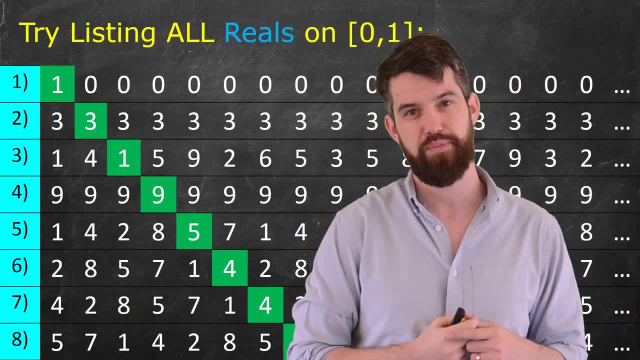 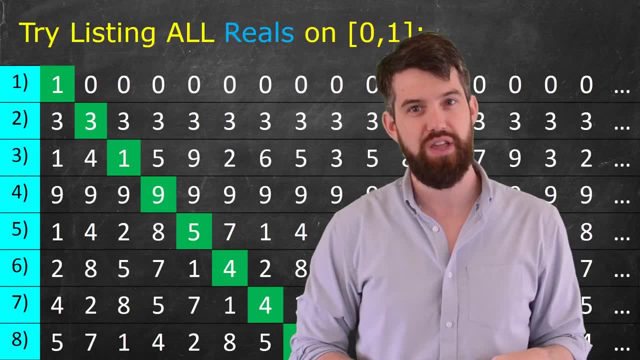 fourth digit in the fourth real number, and so on. It's this diagonal that we have here. What I'm going to do is I'm going to make a new real number that tweaks along this diagonal. So the 1 that we have here. I'm going to go and change that 1 and make it a 2.. Then I look at the 3 that we have. 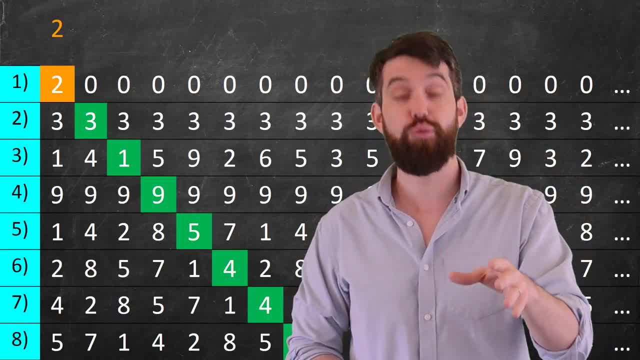 that's in the second row, in the second location. and the 3,: I'm going to add 1 to it and make it a 4.. The 1,: I'm going to go and add 1 to it and make it a 2.. 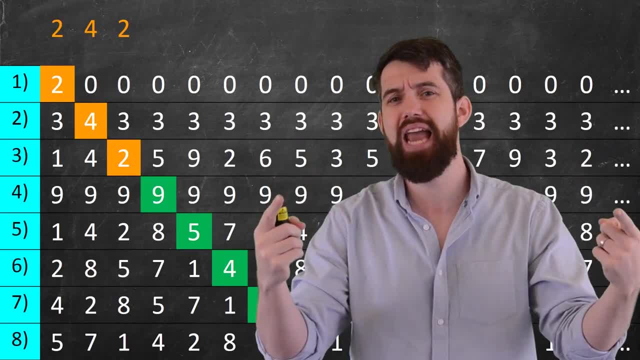 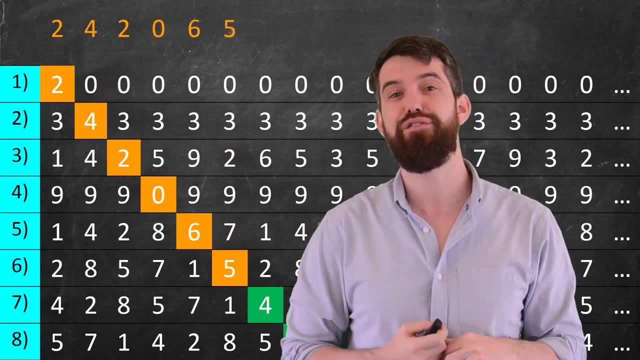 The 9,, I'm going to add 1, but instead of making it a 10,, I'm going to cycle around and make it a 0. So the 9 is going to become a 0,, the 5 is going to become a 6,, the 4 is going to become a 5,. 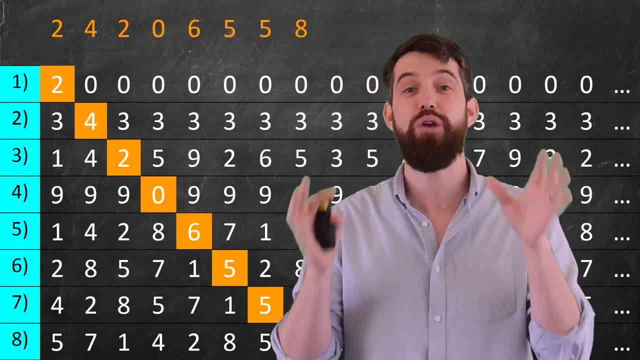 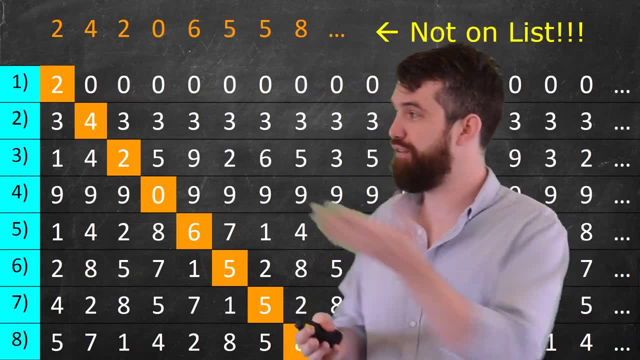 the 4 is going to become a 5, and the 7 is going to become an 8.. And what we have here is a new real number. This real number is not on the list. It's different from the first one. it's different. 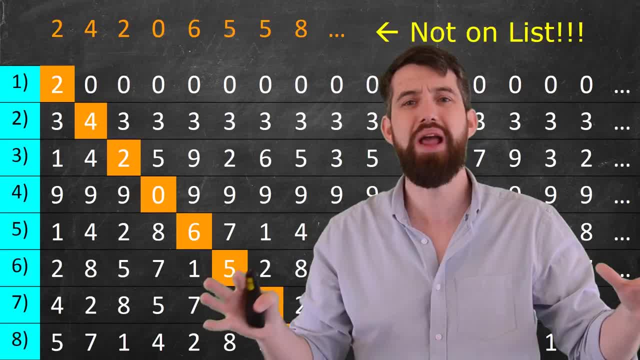 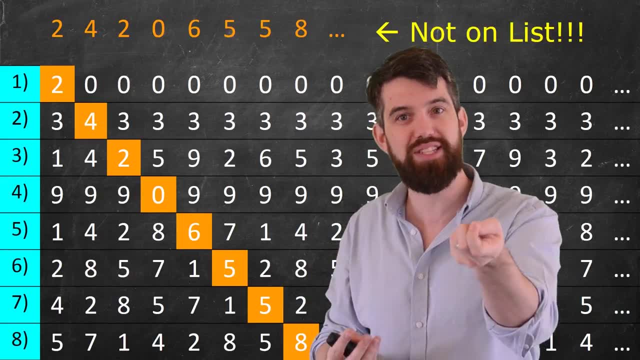 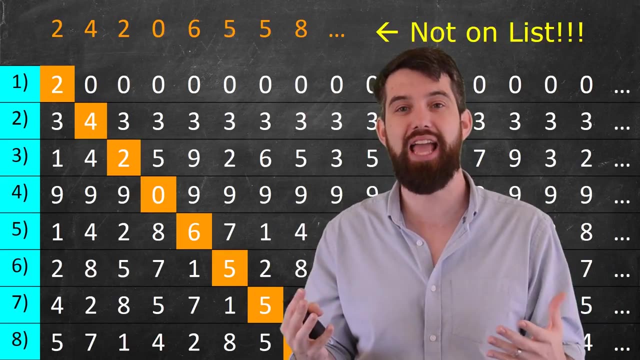 from the second. it's different from the third, So, no matter how you went about choosing your list of numbers, we can always construct this new real number that's different from whatever listing you might have given, And so this tells us that it is not possible to find a function from the integers. 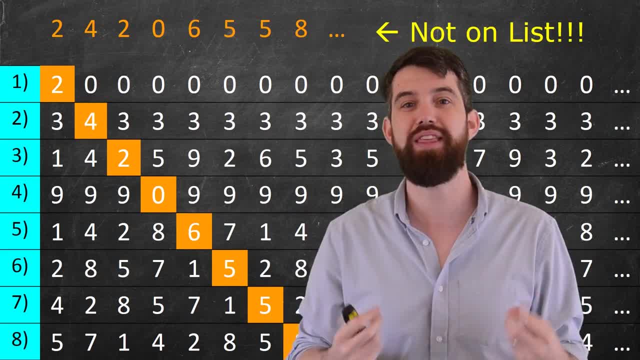 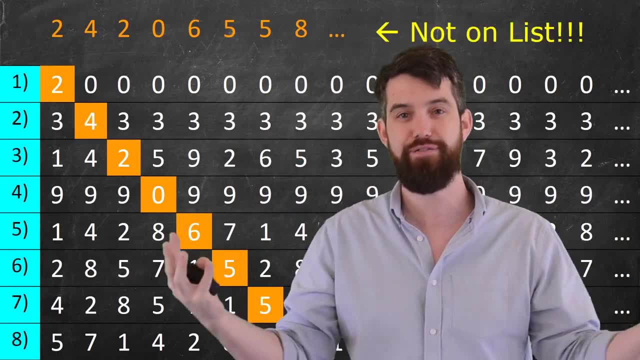 to the real numbers. that has this property that every real number gets listed exactly one time in association with the integers. There's not a bijective function between them, And so what this says in truth is that the integers and the real numbers that they have a 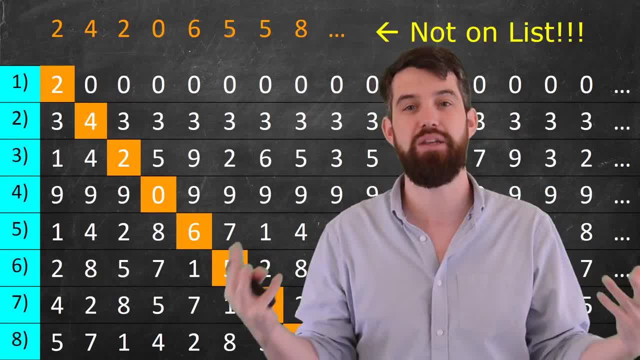 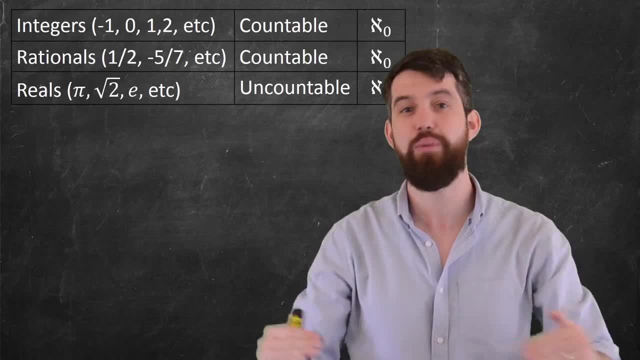 a different size, that you cannot align them in this way. Now we have some terminology for this. When you have an infinite set and you can line it up with the integers where there's a first, a second, a third and so on, we're going to say they're countable because you can align them with. 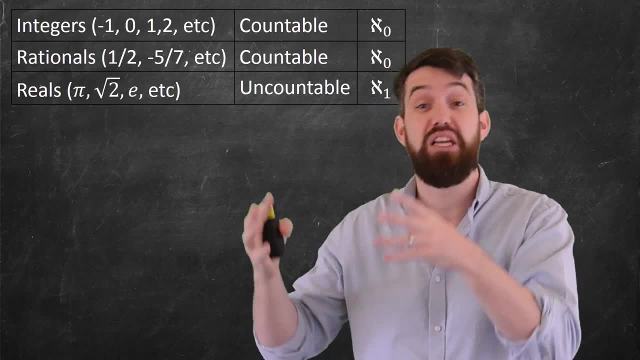 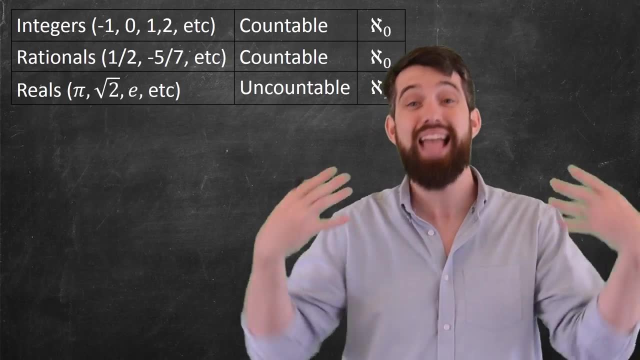 the counting numbers, and there's a fancy math symbol called alif-naught for it, And so what we saw in the first cool math series video was that the rationals were countable, they were alif-naught, and so you could line them up in this way: You could say that there was a first, a second, a third.